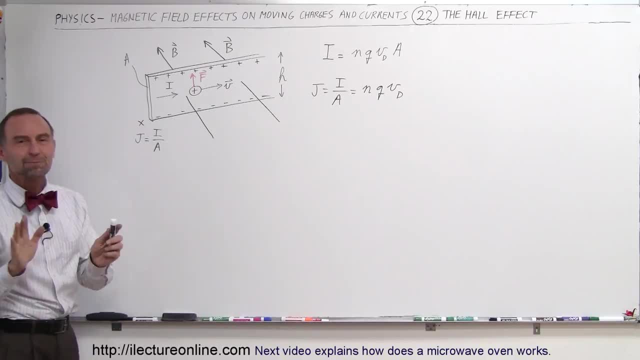 if there's a magnetic field moving from left to…. Oh wow, If there's a magnetic field moving, perpendicular or not moving, but situated perpendicular to the conductor, and there's charges moving in this direction, notice is when these charges are moving in this direction and those move into the left. 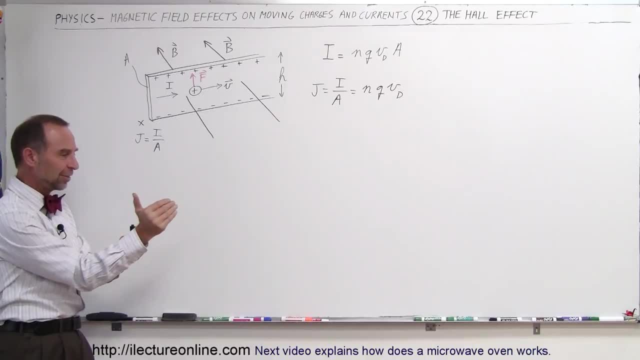 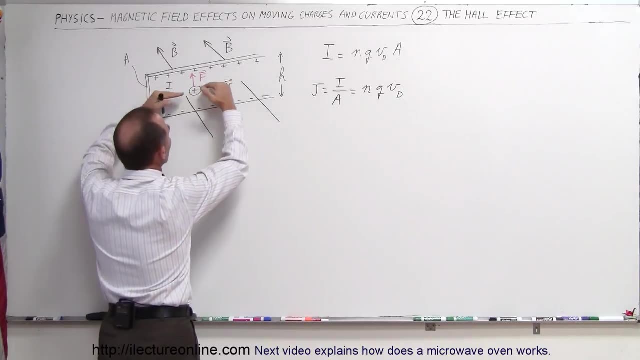 direction. they're positive charges, so we use our right hand and the magnetic field is into the board. that means the force experience is going to be upward, which is drawn right there, and so positive charges would tend to drift towards the top of the conductor and therefore there'll be an excess of. 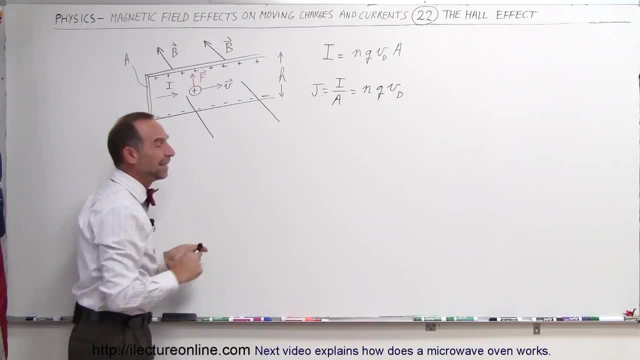 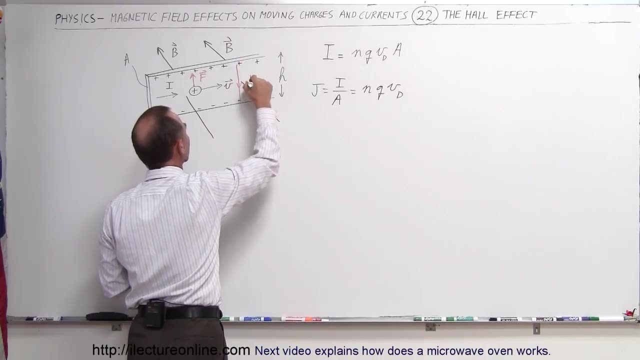 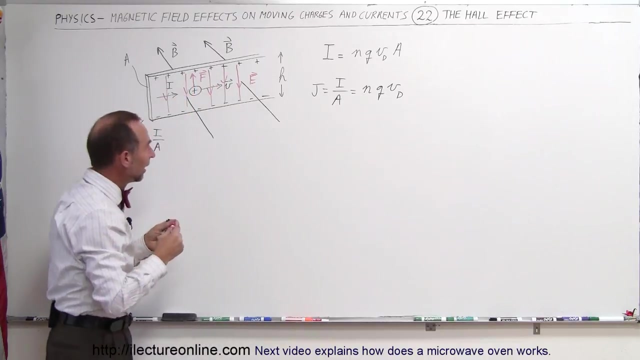 negative charge at the bottom, so there's a separation of charge here. That separation of charge will set up an electric field, so we'll have an electric field then from top to bottom in this direction, all the way through this conductor, and this will be present everywhere, like that. and so what then? 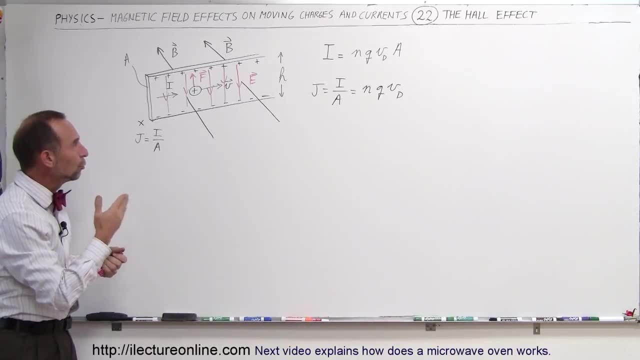 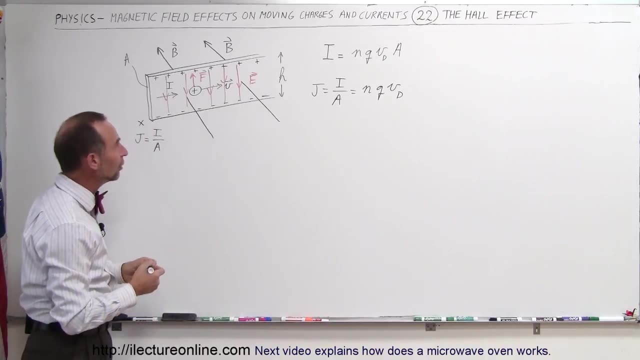 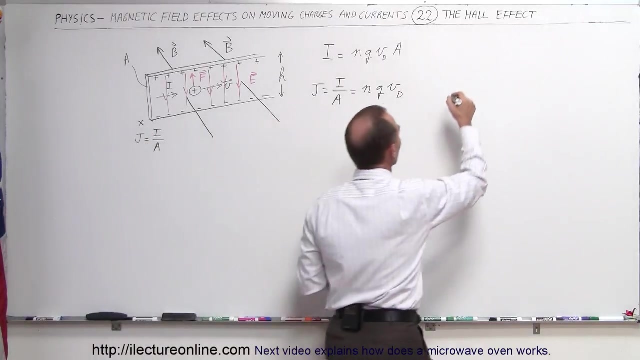 happens is we can then equate the velocity to the strength of the electric field into the strength of the B field. and let's see how we can do that. Well, first of all, the the effect of the magnetic field, of force, of the magnetic field on the moving charges, as follows: force is equal to QVB. and then we also 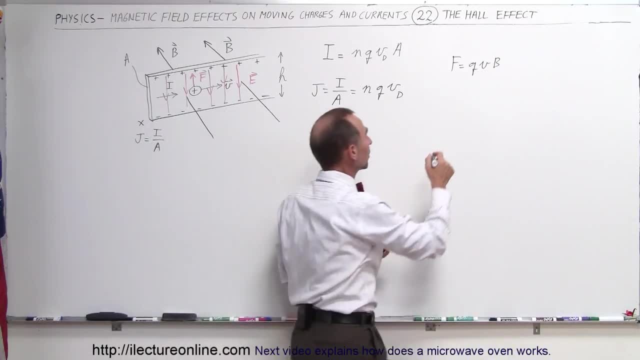 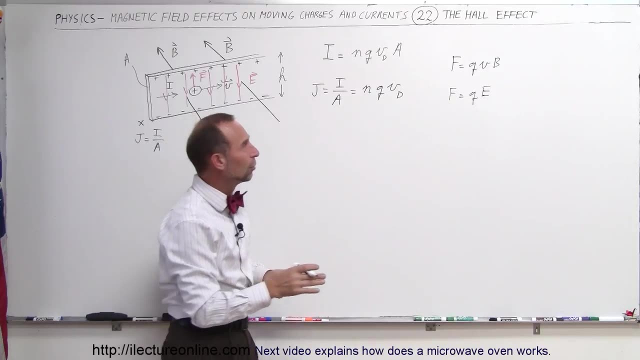 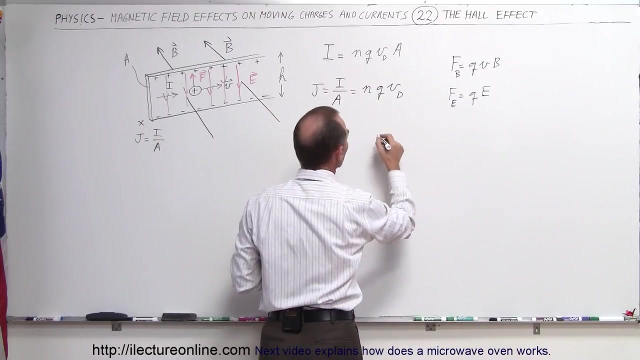 know that the force caused by an electric electric field on the charged particle can also be written as q times the strength of the electric field. So we know that those two forces must be equal. So the force of the magnetic field must be equal to the force caused by the electric field. So therefore we can equate those two equal to. 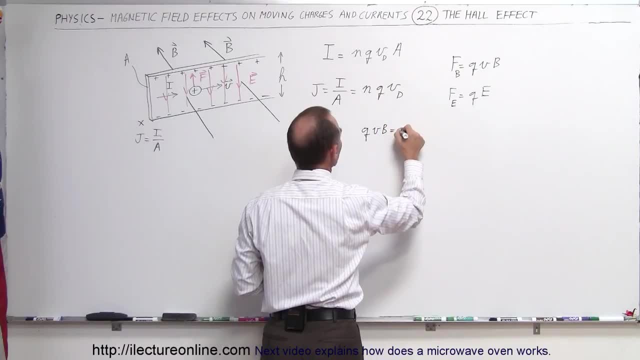 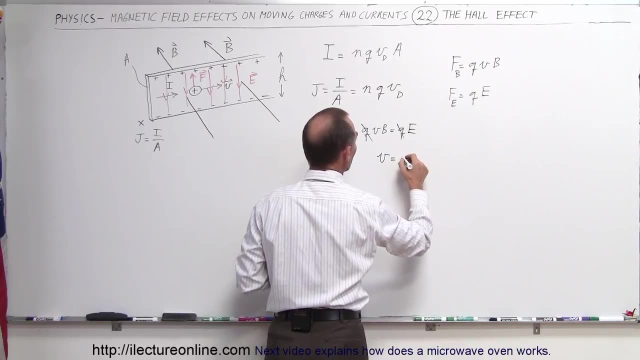 each other. So we can say that q VB must therefore equal to q times E. Notice that the q's cancel on both sides. So we know that the velocity of the charges in there are equal to E divided by B, which is actually interesting when you think about it. That's the same equation that we find. 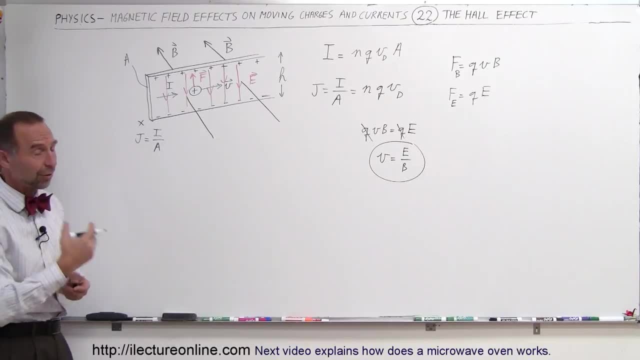 in a velocity selector. And then, of course, is the drift velocity of the charges moving through the conductor. So if we now want to compare the, if we now want to seek out the number of charges that are moving to the top of this conductor in this Hall effect, how do we do that? Well, we know. 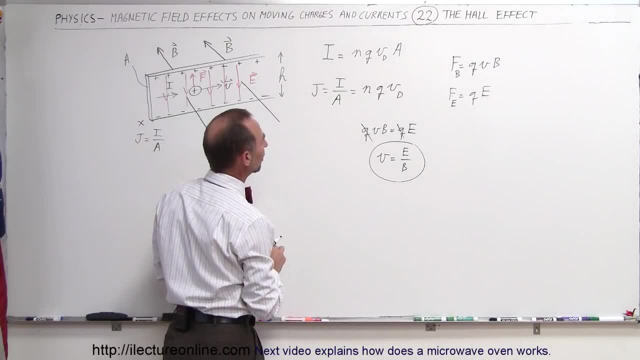 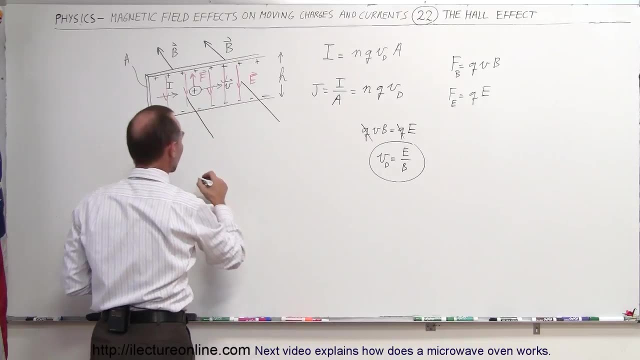 that the current is nq, VD times the cross-sectional area. So there's a relationship between this V right there- This is the drift velocity- and this V right there. So let's write that equation down. We know that the current I is. 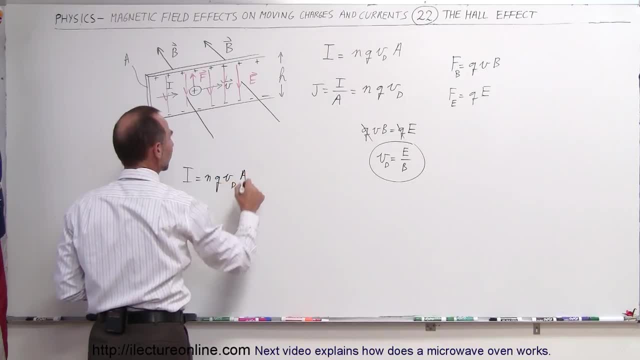 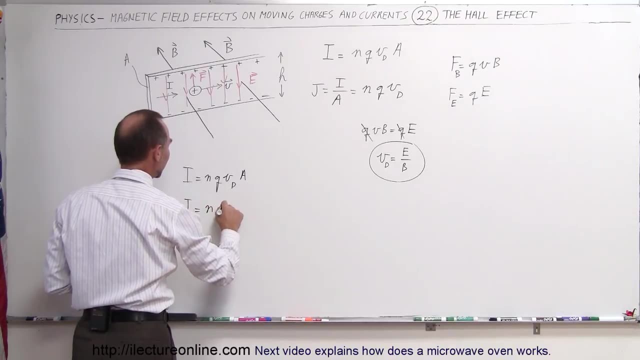 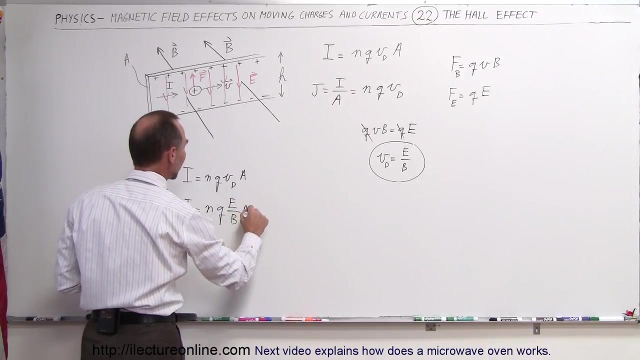 equal to nq V drift times cross-sectional area, And we know that the drift velocity can also be written as E divided by B. So I is equal to n times q times E divided by B. the electric field strength divided by the magnetic field strength times area. Now notice: the magnetic field strength is: 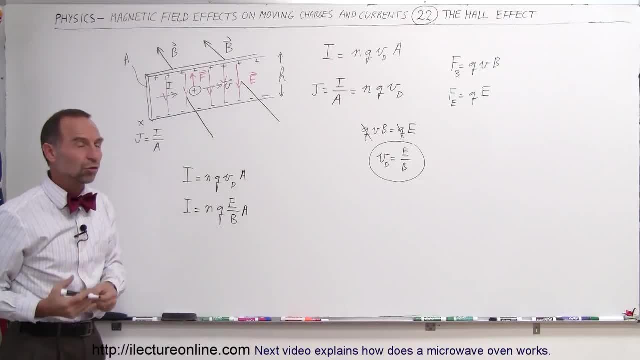 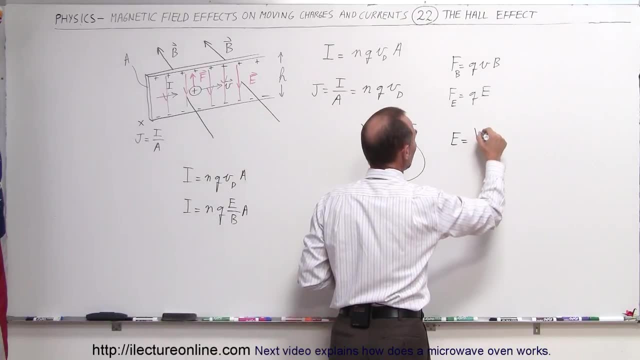 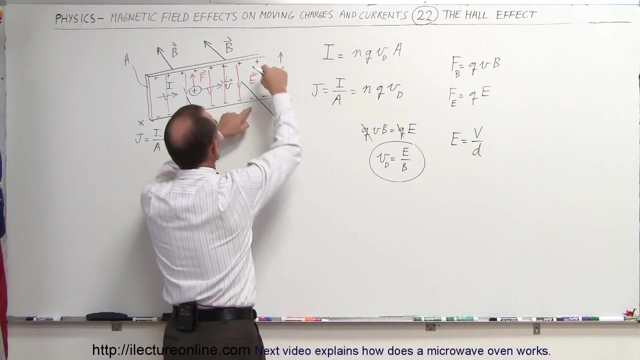 something we know because we apply a certain magnetic field with a certain known strength to that conductor. The electric field can be found by knowing that the electric field can be defined by the potential difference divided by the distance. The distance here will be h and the potential difference is simply something we can measure. We can put two probes on here, and 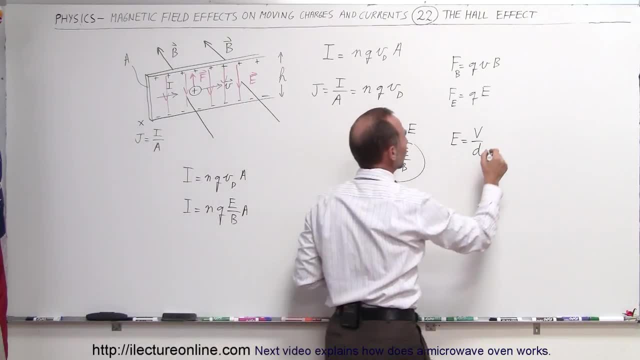 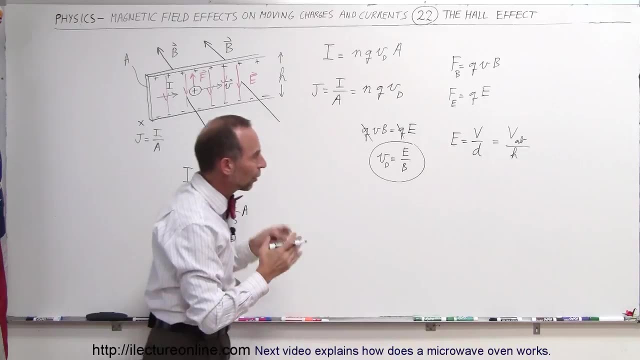 measure the potential difference between the top and the bottom of the conductor. So this can be measured to be V between A and B, the top and the bottom divided by h, which is the height of the conductor or the distance between one end and the other end. So those are two measurable values. 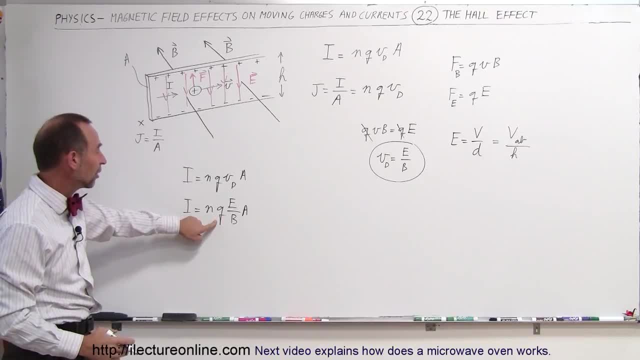 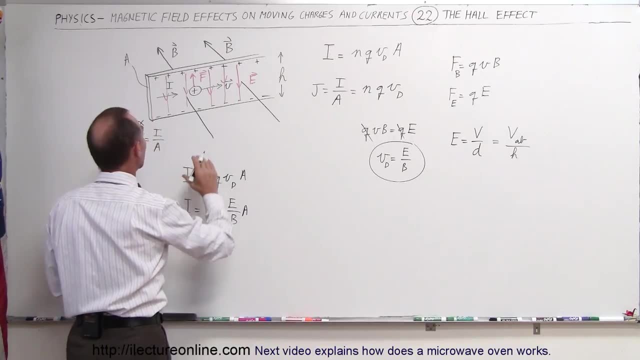 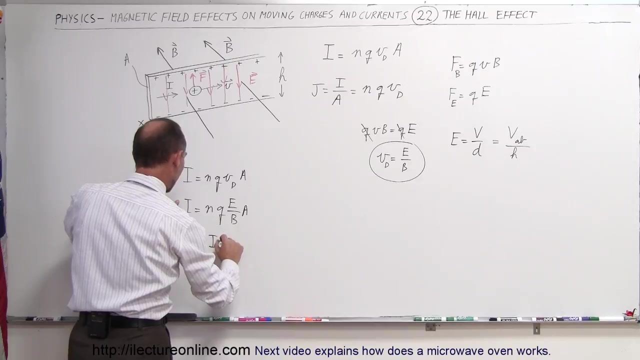 We can assume the charge to be a single unitary charge and we can measure the cross-sectional area. So therefore we can see that n the number of charges per unit volume that move to the top of this due to the Hall effect is going to be equal to. we have I times B divided by. let's see here we have: 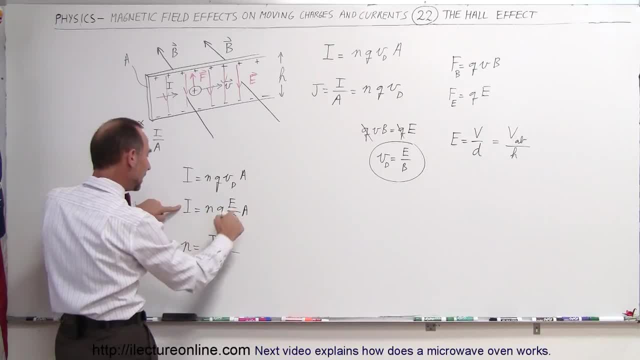 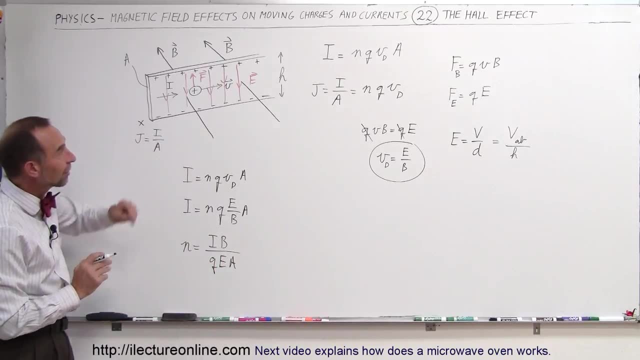 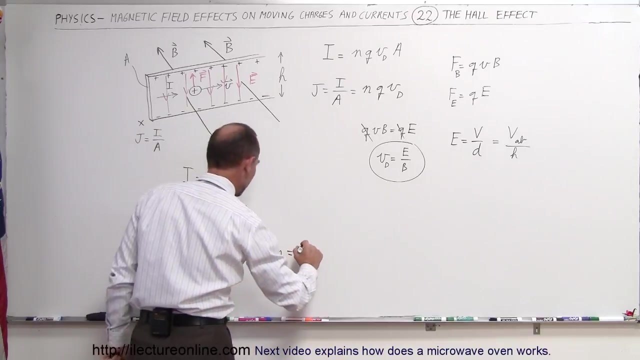 I and B to the top, nq e and A. so we have nq e and A to the bottom and of course we can then say that the current density is I divided by A. so we can say that the number of charges per unit volume that move to the top can be expressed in: 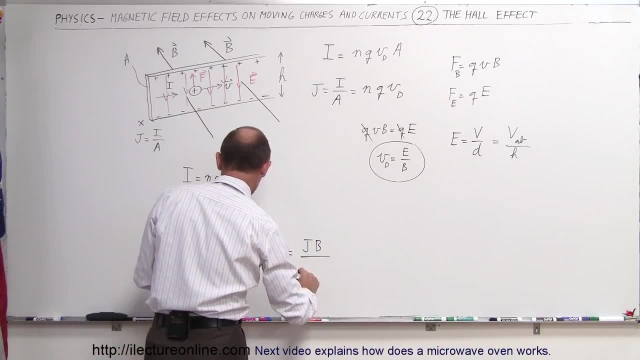 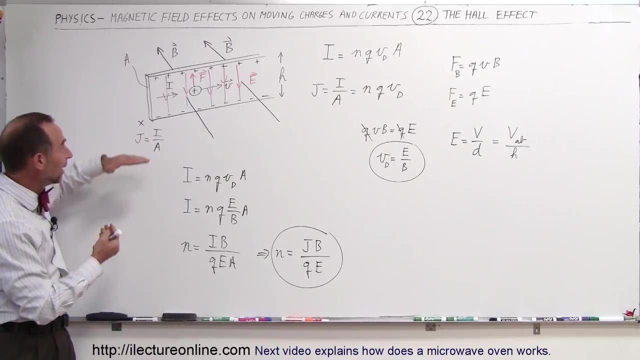 terms of the current density, times the magnetic field, divided by the size of each charge, times the electric field. And that's how Hall determined two ways: One, that the charges, he could determine the type of charge that move into the conductor, depending upon how the potential difference is. 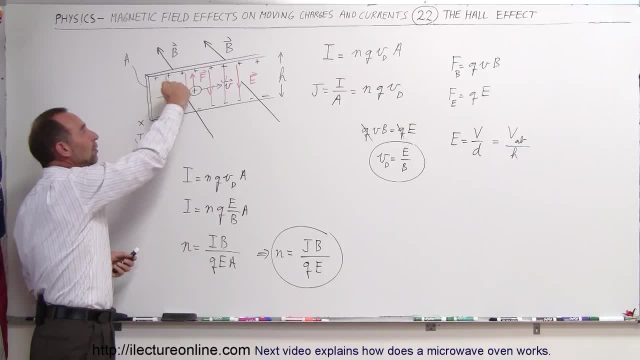 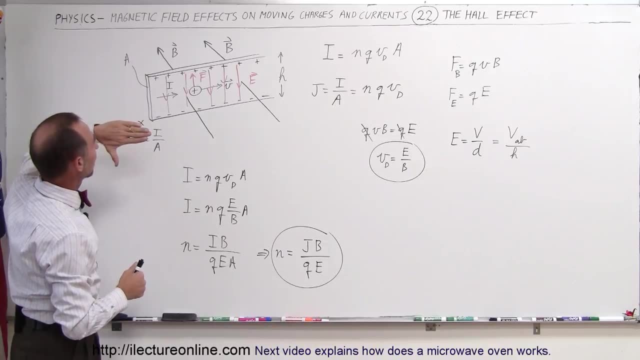 set up. For example, if these were negative charges, they would then be moving to the bottom, and so you get this differentiation like that. Let's see here Negative charges, B field, negative charges moving this way. so, yeah, the negative charges would be moving this way.